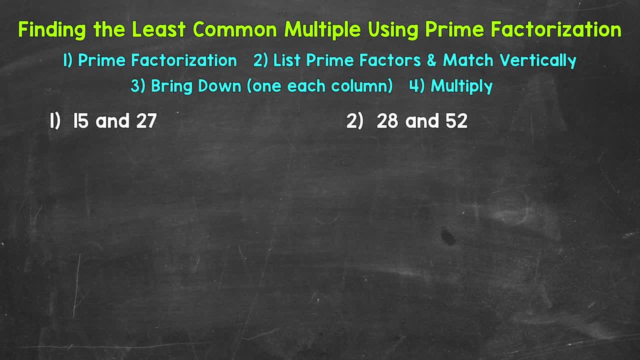 common multiple. Let's jump into our examples, starting with number 1, where we have 15 and 27.. Let's start with the prime factorization of 15, and we will start with the factors of 3 and 5.. 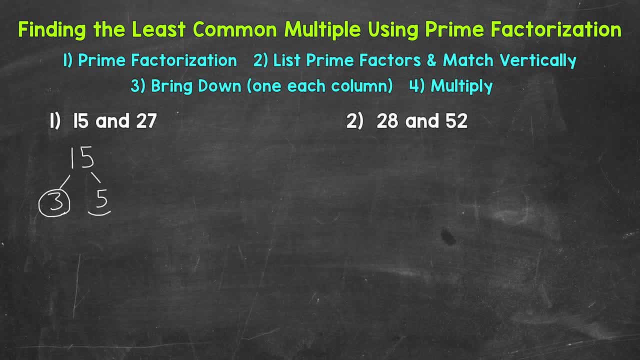 Now, 3 is prime, so we are done there, and 5 is prime, so we are done there as well, And that's the prime factorization of 15.. We can't break that down any further. Now we have the prime. 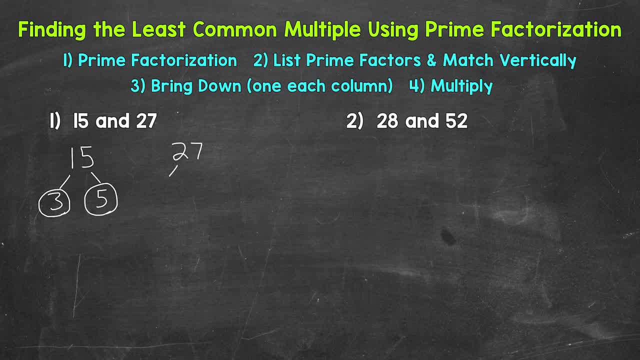 factorization of 27.. Let's start with the prime factorization of 15, and we will start with the factors of 3 and 9.. 3 times 9 equals 27,, so 3 and 9 are factors of 27.. 3 is prime, so we are done. 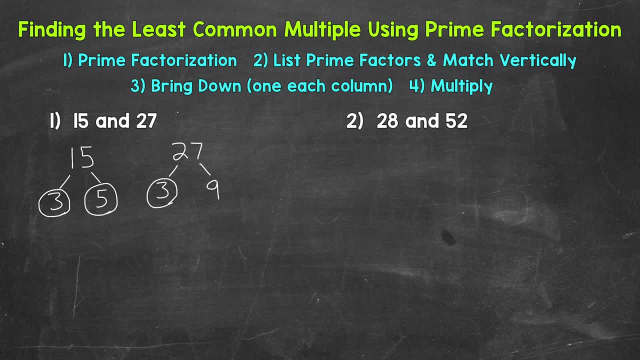 there. but we can break 9 down 3 times 3 equals 9, so 3 is a factor of 9.. 3 is prime. so we are done there and there. Let's start with the prime factorization of 27.. We can't break that down any further Now. we're. 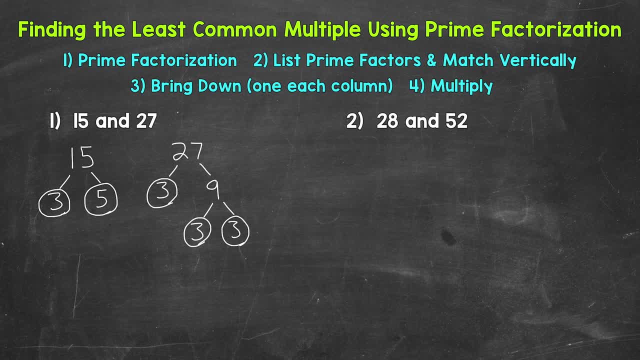 ready to move to the next step. So we need to list the prime factors of 15 and 27 and match them vertically. Let's see what this looks like, starting with 15.. So our prime factors from the prime factorization are 3 and 5, or 3 times 5.. Now 4.. 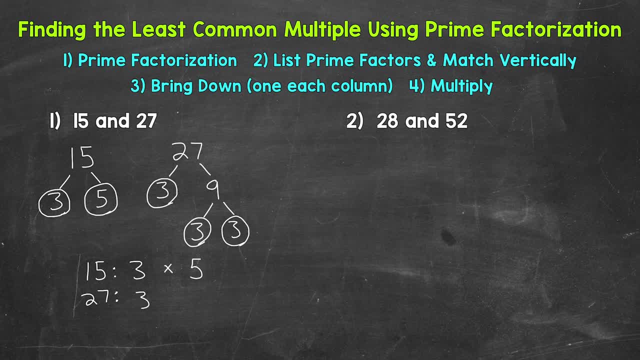 27.. So we have 3 times 3 times 3.. And you'll notice that big gap underneath the 5. there We are matching numbers vertically. 27 does not have a prime factor of 5, so I left that blank underneath. 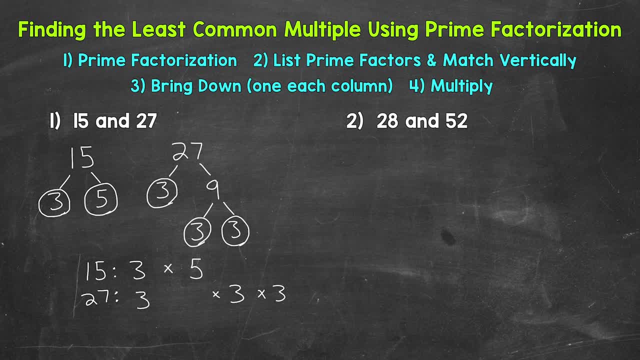 the 5.. Now that we have our prime factors listed and matched vertically, we move on to the next step, where we break down the prime factors. So we have 3 times 3 times 3 times 3.. And you'll notice. 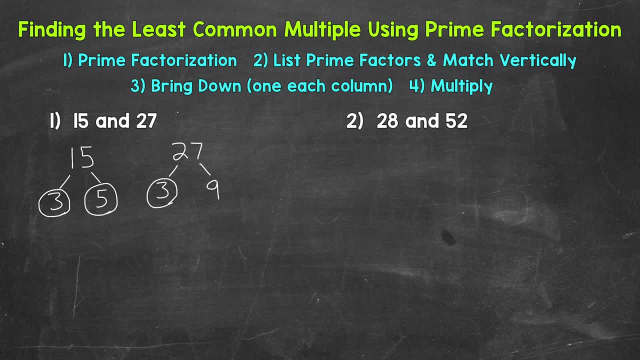 there. but we can break 9 down 3 times 3 equals 9, so 3 is a factor of 9.. 3 is prime. so we are done there and there. Let's start with the prime factorization of 27.. We can't break that down any further Now. we're. 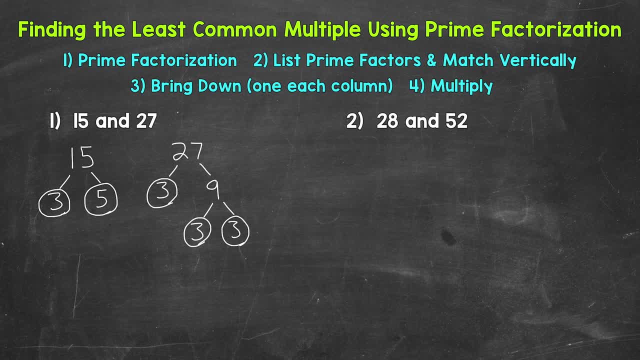 ready to move to the next step. So we need to list the prime factors of 15 and 27 and match them vertically. Let's see what this looks like, starting with 15.. So our prime factors from the prime factorization are 3 and 5, or 3 times 5.. Now 4.. 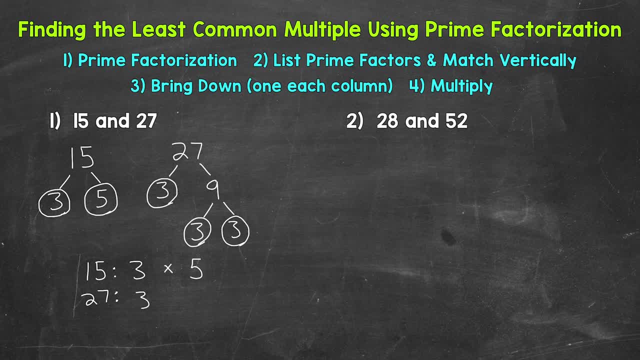 27.. So we have 3 times 3 times 3.. And you'll notice that big gap underneath the 5. there We are matching numbers vertically. 27 does not have a prime factor of 5, so I left that blank underneath. 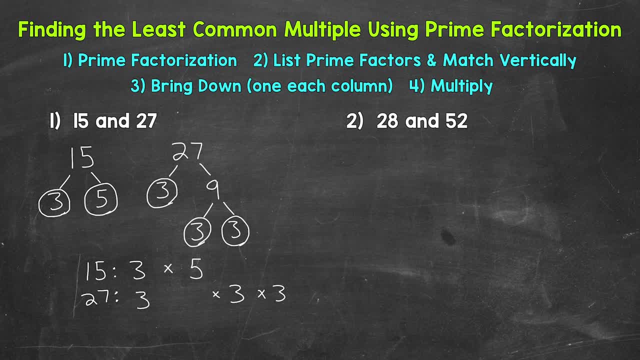 the 5.. Now that we have our prime factors listed and matched vertically, we move on to the next step, where we break down the prime factors. So we have 3 times 3 times 3 times 3.. And you'll notice. 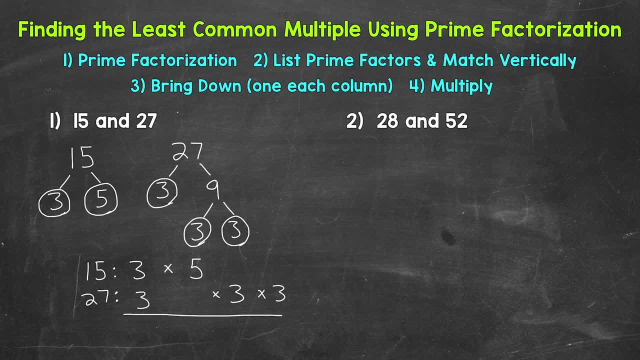 that second time that 3 is here, 2 times 3 times 3 times 3.. And that is what this golľab 1 is 1, so it's 2 times the final value of each of these prime factors. 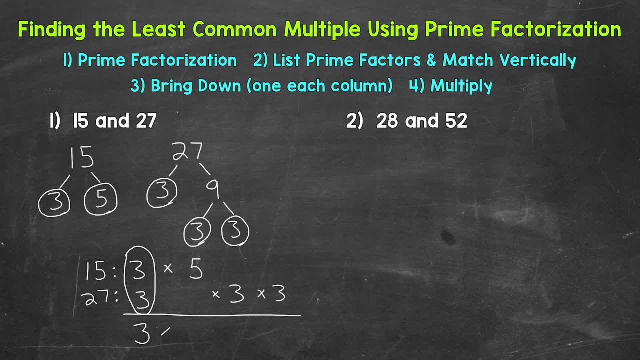 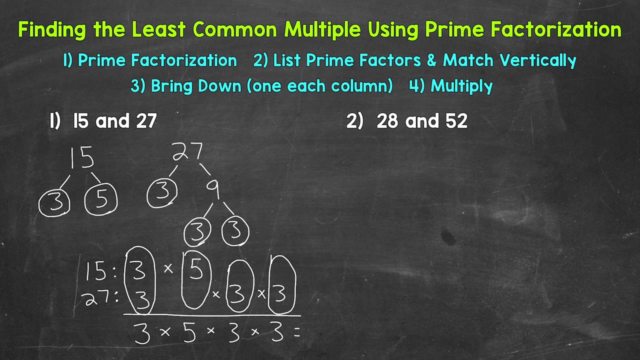 27 is of course 20.. 22 is prime of 3 times 5. Which I needahan value of 2 times 2 x 3, Значит mit 3.. here times another 3 here. So we end up with 3 times 5 times 3 times 3.. And by multiplying these, 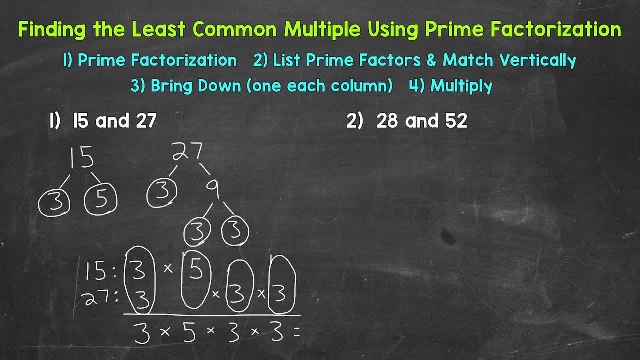 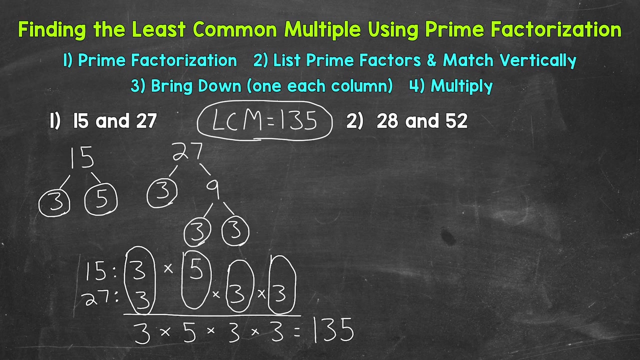 we get our least common multiple. So 3 times 5 is 15, times 3 is 45, times 3 is 135.. And that's our least common multiple. So the LCM, the least common multiple of 15 and 27, is 135.. Let's move. 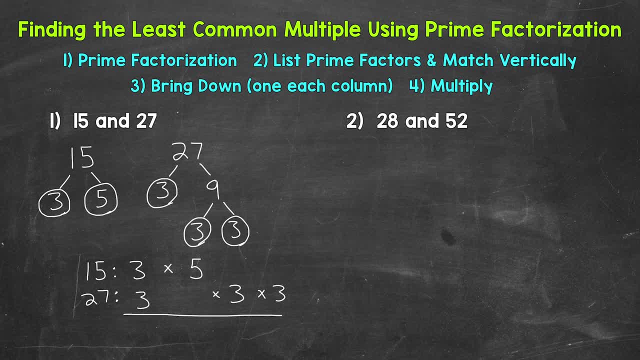 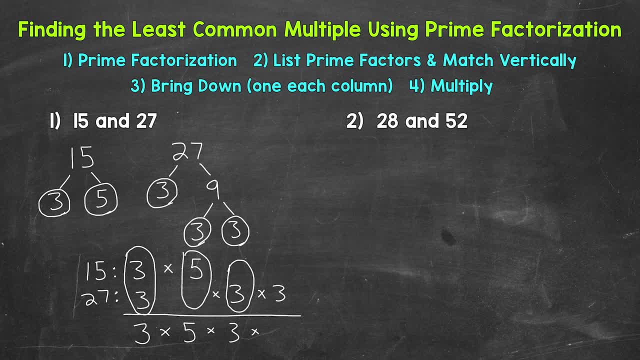 Oh, there we go. I'm not sure why I did that. Oh there we go. Oh there we go. Oh there we go here. times another 3 here, So we end up with 3 times 5 times 3 times 3.. And by multiplying these, 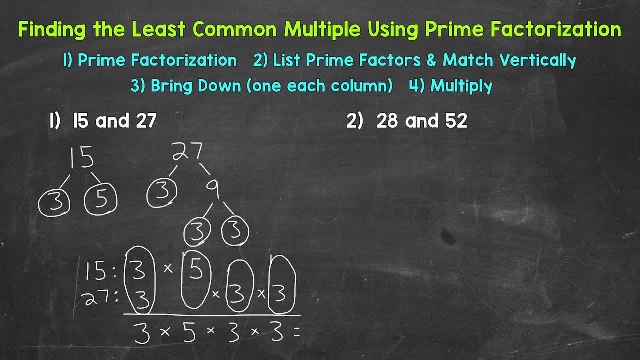 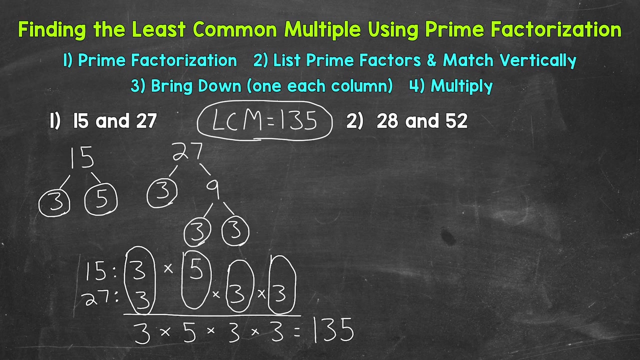 we get our least common multiple. So 3 times 5 is 15, times 3 is 45, times 3 is 135.. And that's our least common multiple. So the LCM, the least common multiple of 15 and 27, is 135.. Let's move. 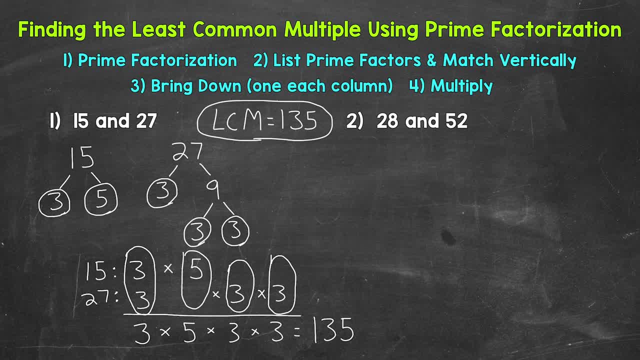 on to number 2, where we have 28 and 52. Let's start with the prime factorization of 28.. Now, 2 times 14 equals 28.. So let's start with those factors. 2 is prime, So we are done there. 14, we can break down 2 times 7, equals 14.. So 2 and 7 are factors of 14.. 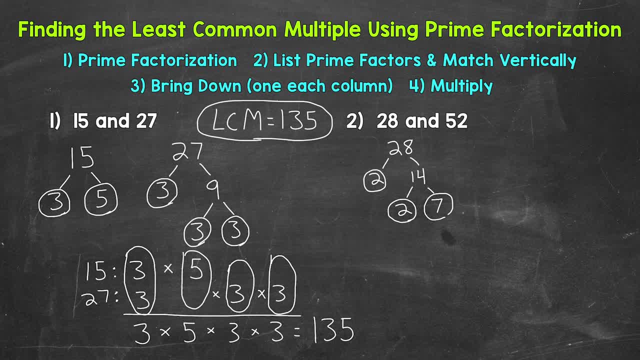 2 is prime, So we are done there. And 7 is prime as well, So we are done there, And that's the prime factorization of 28.. We can't break that down any further Now. we need the prime factorization. 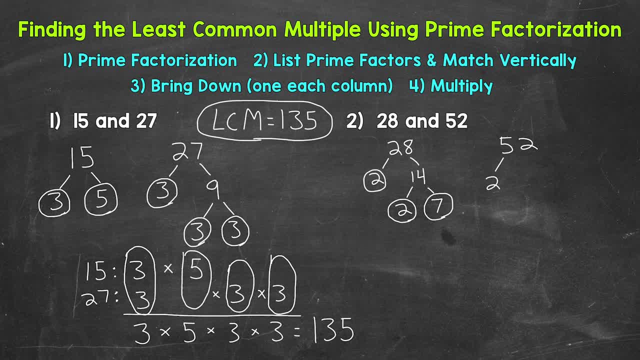 of 52.. Let's start with the factors of 2. And 26.. 2 times 26 equals 52.. So 2 and 26 are factors of 52.. 2 is prime. So we are done there. 26, we can break that down- 2 times 13, equals 26.. So 2 and 13 are factors of 26.. 2 is prime. 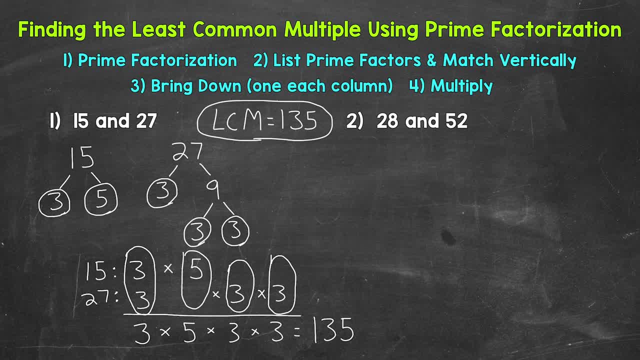 on to number 2, where we have 28 and 52. Let's start with the prime factorization of 28.. Now, 2 times 14 equals 28.. So let's start with those factors. 2 is prime, So we are done there. 14, we can break down 2 times 7, equals 14.. So 2 and 7 are factors of 14.. 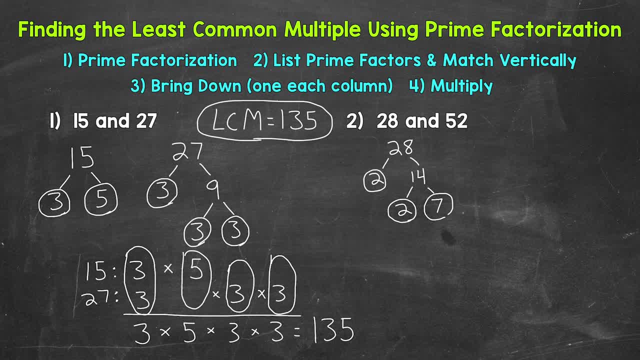 2 is prime, So we are done there. And 7 is prime as well, So we are done there, And that's the prime factorization of 28.. We can't break that down any further Now. we need the prime factorization. 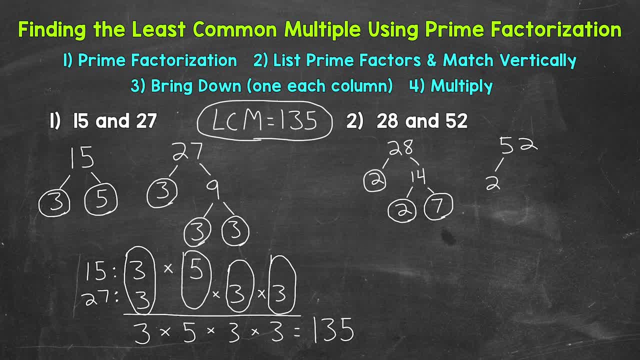 of 52.. Let's start with the factors of 2. And 26.. 2 times 26 equals 52.. So 2 and 26 are factors of 52.. 2 is prime, So we are done there. 26, we can break that down- 2 times 13, equals 26.. So 2 and 13 are factors of 26.. 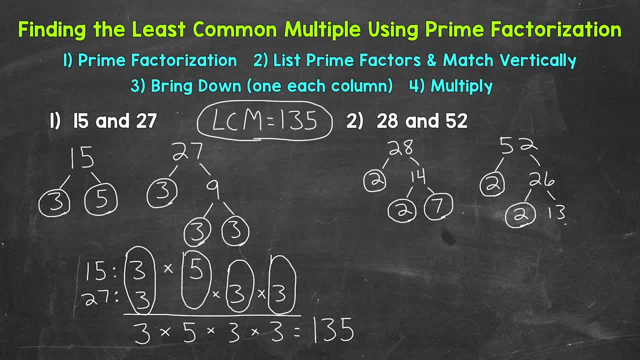 2 is prime, So we are done there. And 13 is prime as well, So we are done. And that's the prime factorization of 52.. We can't break that down any further. Now we need to list the prime factors and match them vertically. 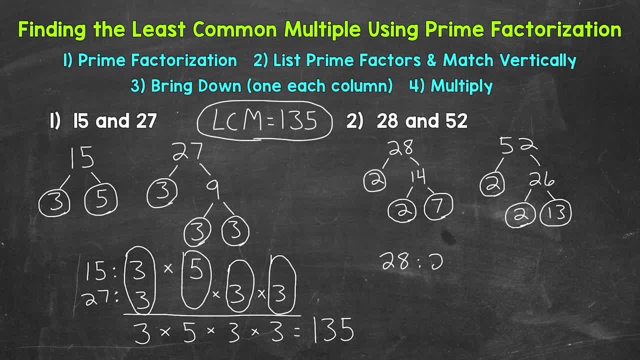 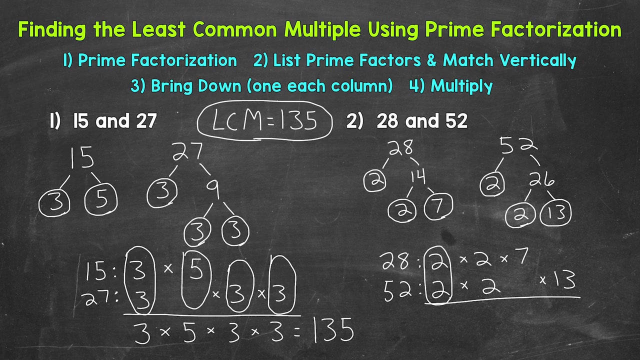 For 28, we have 2 times 2 times 7.. For 52, we have 2 times 2 times 13.. Now we need to bring down. So we have a column of 2s here, So let's bring down a 2 to represent that column. 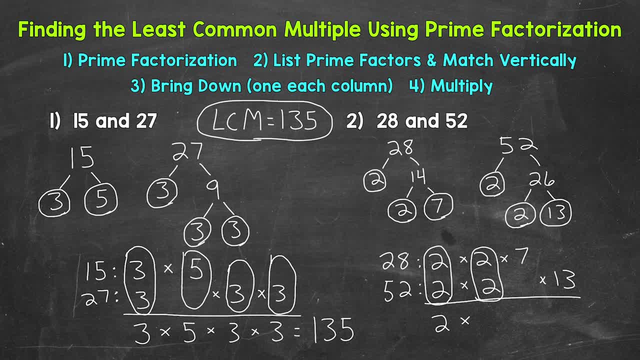 Times, another column of 2s, So let's bring another 2 down. Times 7 times 13.. So we have 2 times 2 times 7.. Times 13, to get our least common multiple. We have 2 times 2,, which is 4.. 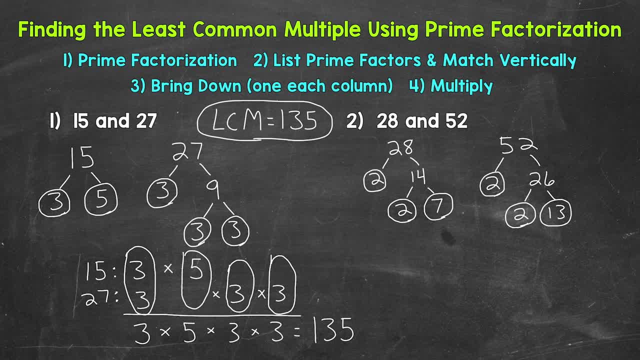 So we are done there, And 13 is prime as well. So we are done, And that's the prime factorization of 52.. We can't break that down any further. Now we need to list the prime factors and match them vertically. 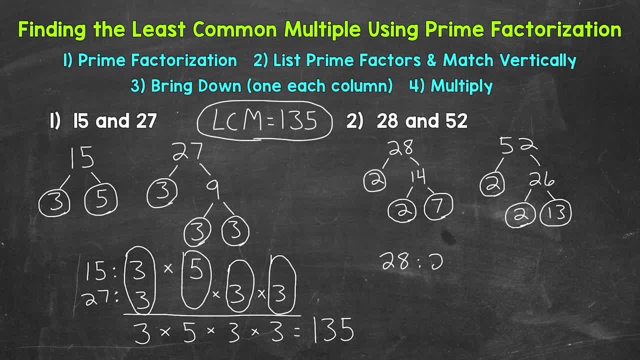 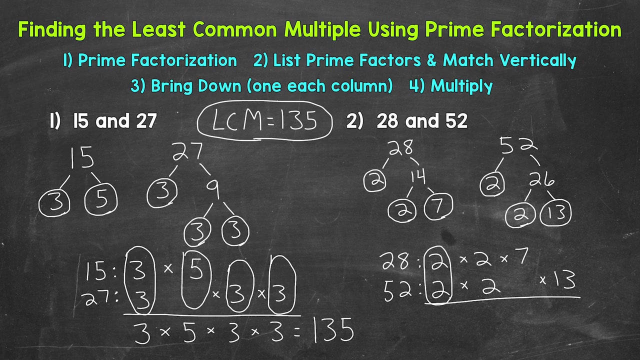 For 28, we have 2 times 2 times 7.. For 52, we have 2 times 2 times 13.. Now we need to bring down. So we have a column of 2s here, So let's bring down a 2 to represent that column. 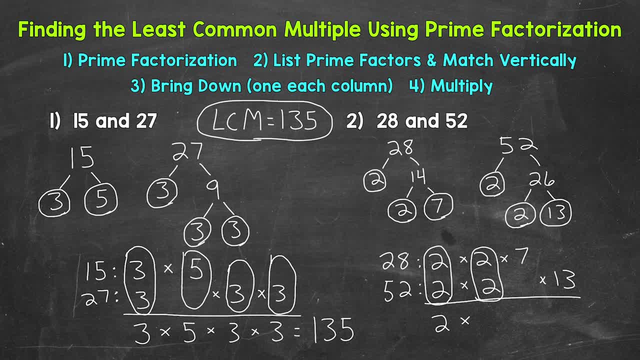 Times, another column of 2s, So let's bring another 2 down. Times 7 times 13.. So we have 2 times 2 times 7.. Times 13, to get our least common multiple. We have 2 times 2,, which is 4.. 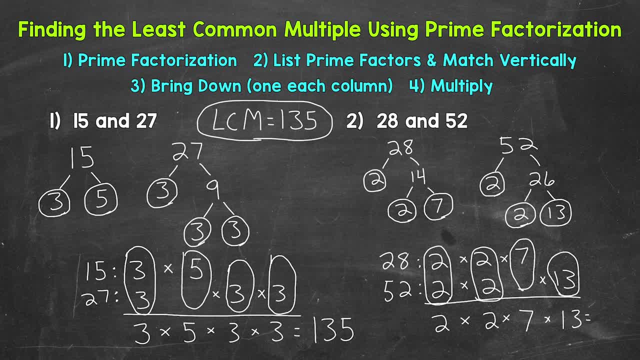 Times 7 is 28.. Times 13.. Well, I'm not sure what 28 times 13 is, So let's come to the side here And multiply 28 times 13.. We will start with 3 times 8, which is 24.. 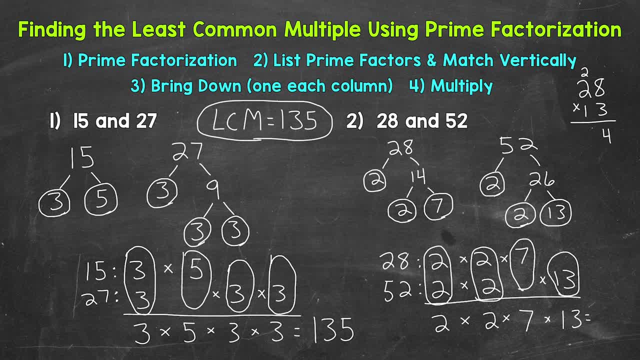 3 times 2 is 6.. Plus 2 is 8.. We are done here and done here. We need a 0.. Now we have 1 times 8, which is 8.. And then 1 times 2 is 2.. 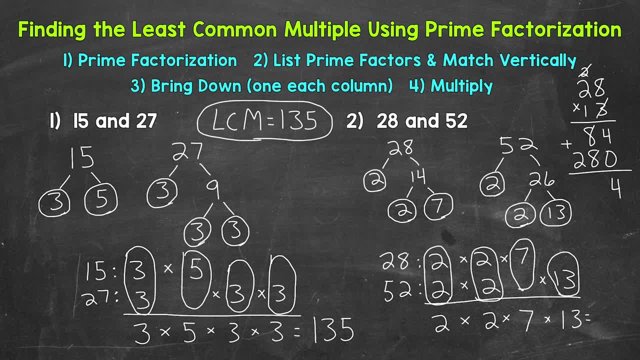 Let's add: 4 plus 0 is 4.. 8 plus 8 is 16.. And then 1 plus 2 is 3.. So we get 364.. So the least common multiple Of 28 and 52, let me squeeze this in here- is 364.. 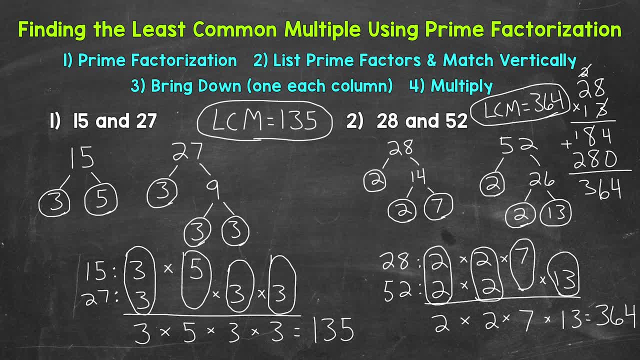 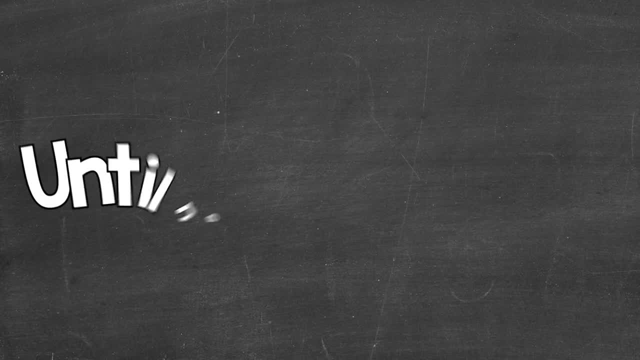 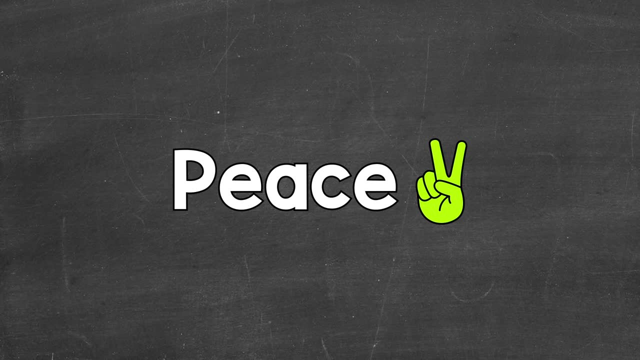 So there you have it. There's how to find the least common multiple using prime factorization. I hope that helped. Thanks so much for watching. Until next time, peace, Bye.